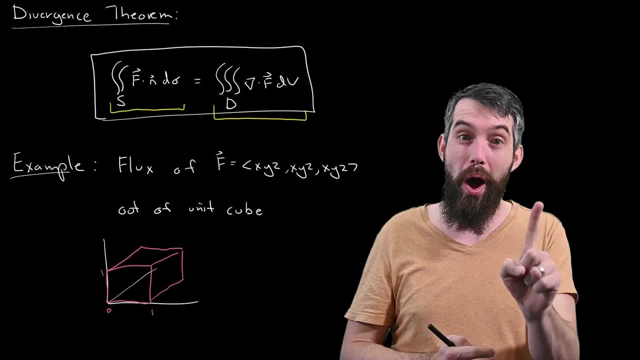 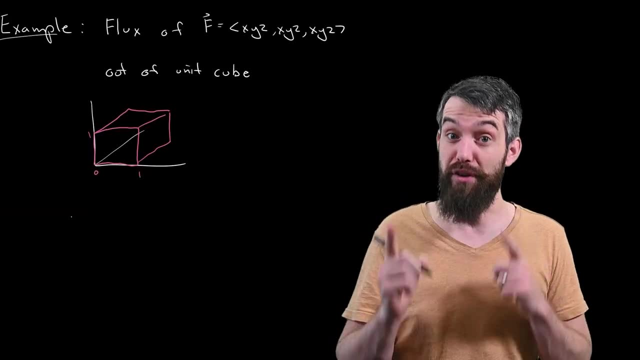 of having six different surface intervals for the six sides, we're going to have one interval that's going to be very easy to compute. So I'm going to use the right side of the divergence theorem, So giving myself a bit more space. the first thing I need to do is compute the divergence of f, So 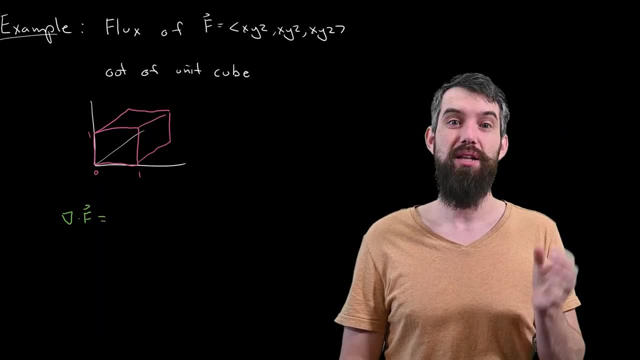 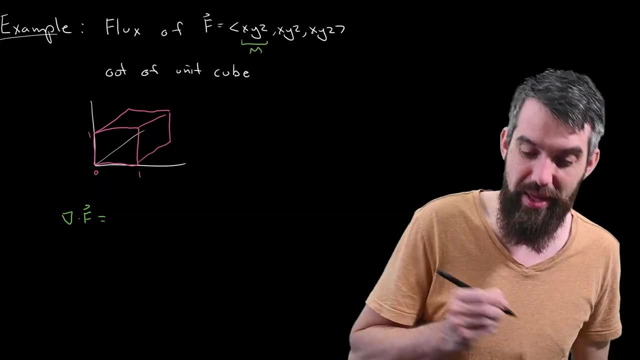 this is the sum of the parts with respect to x of the first component, its parts with respect to y of the second component and the partial respect to z of the third component. So first component- here we'll maybe call it the- m is x, y and z. The partial of that with respect to x is equal to y- z. Then I'm. 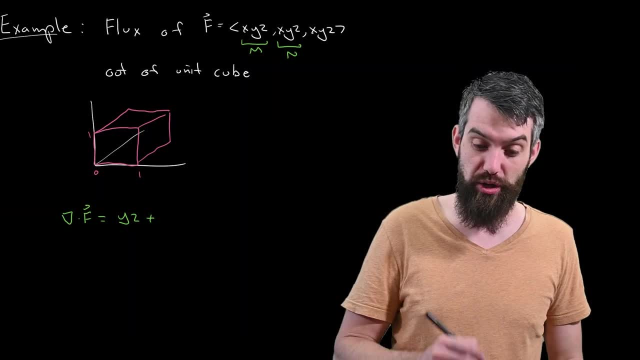 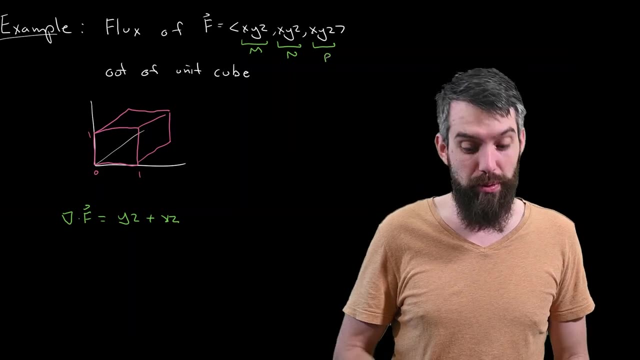 going to take the partial of the second component, which we often call m, partial of that with respect to y, which is going to leave me with an x, z, And then, finally, the third component, which we often call p. partial of p with respect to z is going to give me a x, y, And so what I'm interested in? 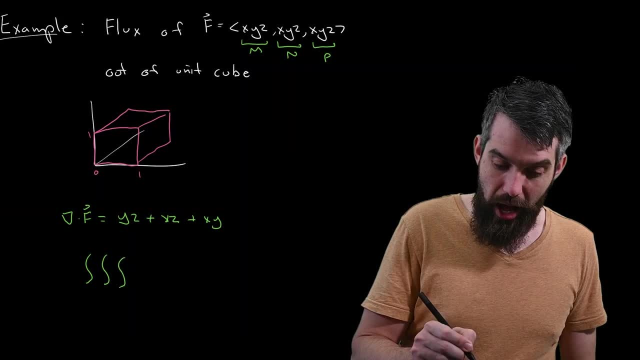 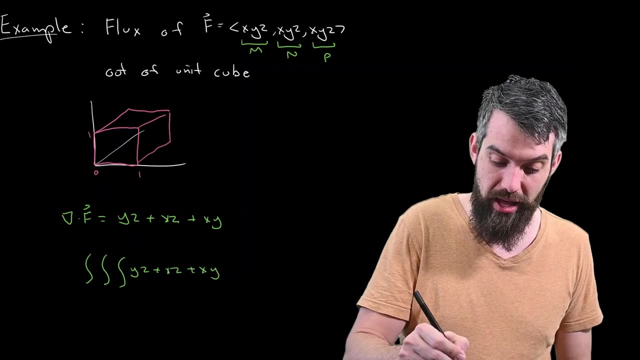 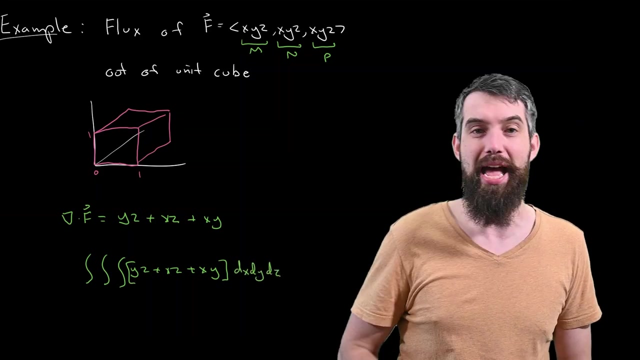 computing then, is the triple integral of this divergence. So I'll just copy and paste y, z plus x, z plus x, y. I'll put that in brackets And then I'm going to do an interval with respect to volume, a little dx, dy, dz In more complicated examples. maybe you're going to care about which. 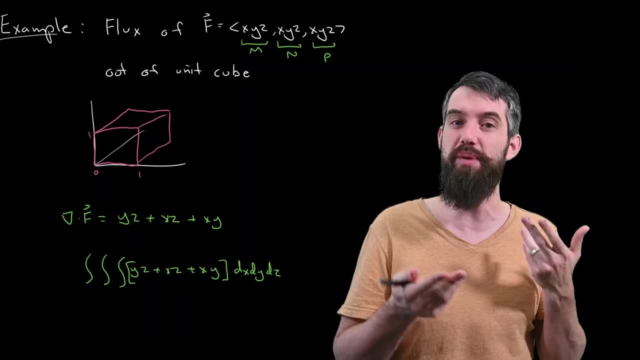 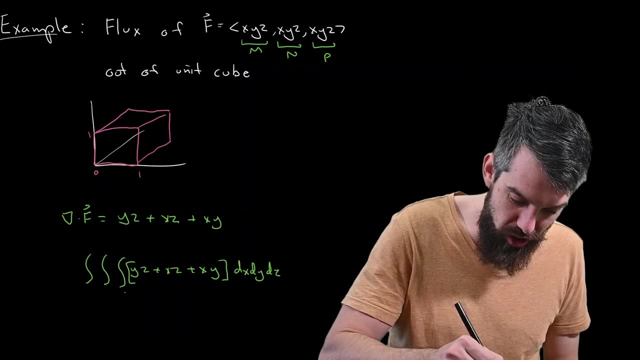 order the dv you do. is it dx, dy, dz or some other permutation? And if the region was easier to describe in terms of the limits one way or the other, you might have a preference. But in here it's the unit cube. So x is going between 0 and 1, y is going between 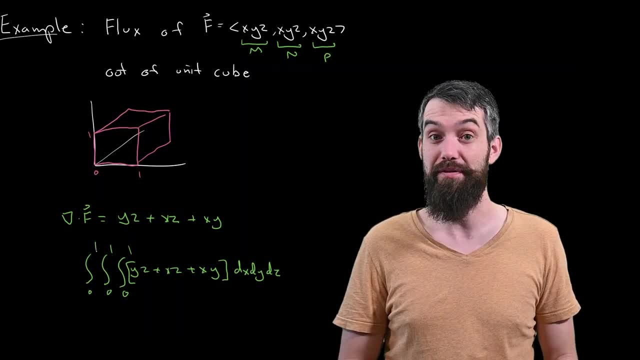 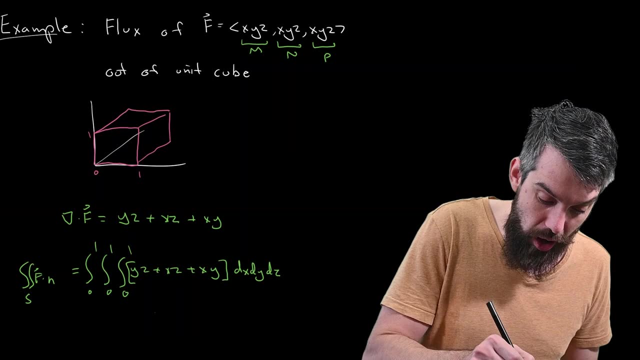 0 and 1, and z is going between 0 and 1.. That's all I get, And by the divergence theorem this entire thing better be equal to that surface integral, the f dot n, d sigma. That is the flux. 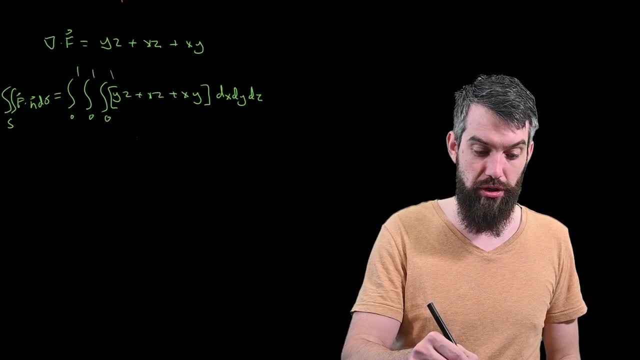 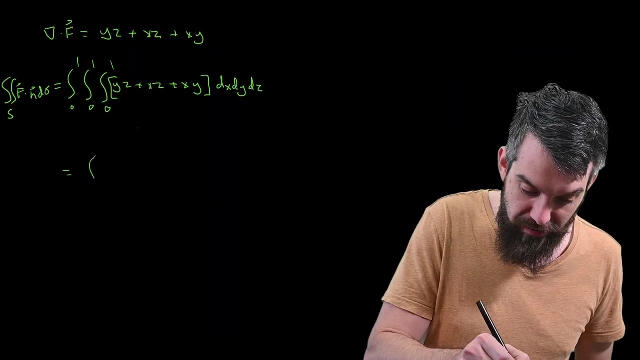 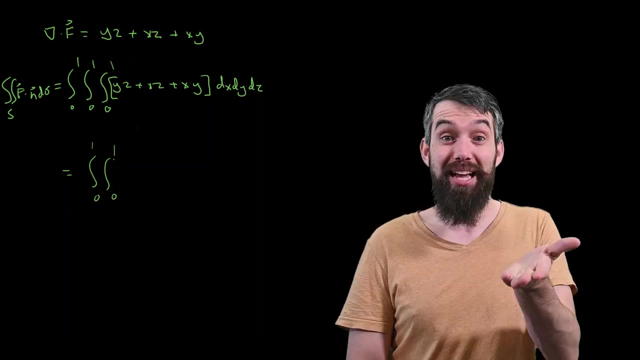 across the cube. Okay, so let's go and try to actually do this computation now. It shouldn't be so bad for us. Well, first I'm going to do the integral with respect to x, So I'll leave the outer two integrals up: 0 to 1 and 0 to 1.. The first term is yz. It integrates to yz times x. 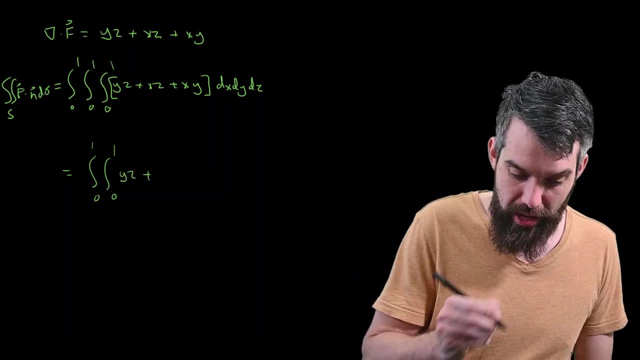 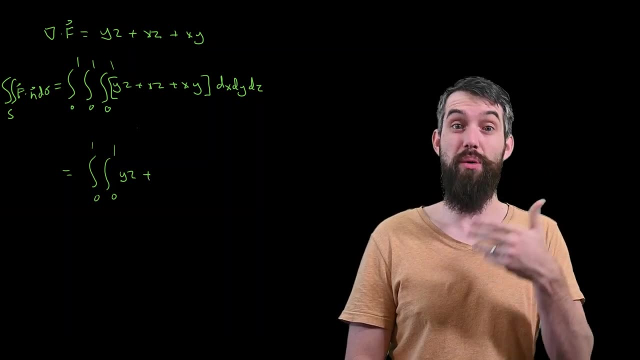 between 0 and 1.. It's just going to give me y times z. There is an x in the second term, so it integrates to x squared over 2 times z And then evaluated between 0 and 1 is just going. 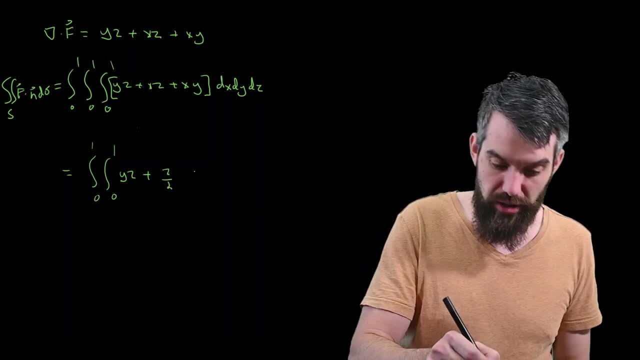 to give me z divided by 2.. And likewise for the third term. here I have an x It's going to integrate to x squared over 2 multiplied by the y Evaluated to 0 and 1, I just get that half. 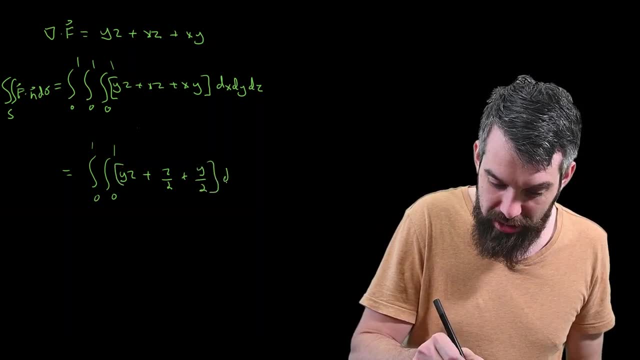 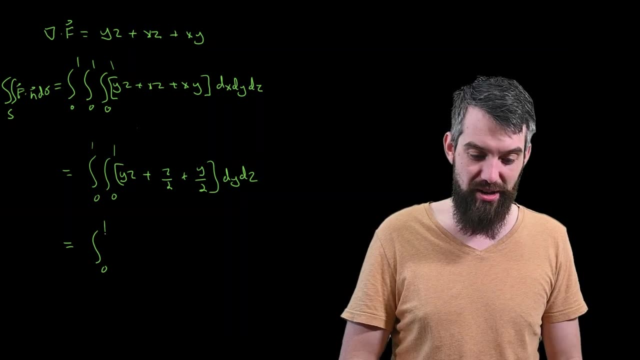 y divided by 2.. And then I've already integrated out the dx, so I just have a dy dz remaining. Let's do the next, most inner integral. So I have just the outside one remaining here. So y now is what has been integrated, so integral with respect to y. So the integral of yz becomes. 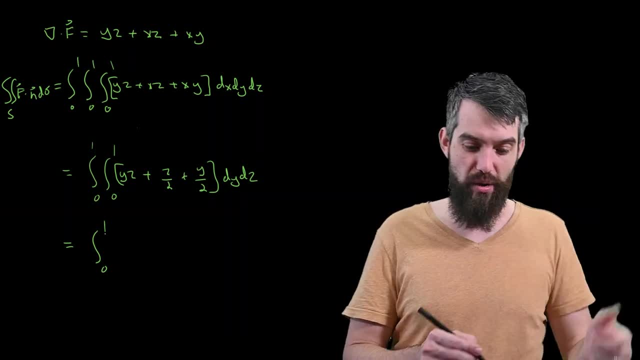 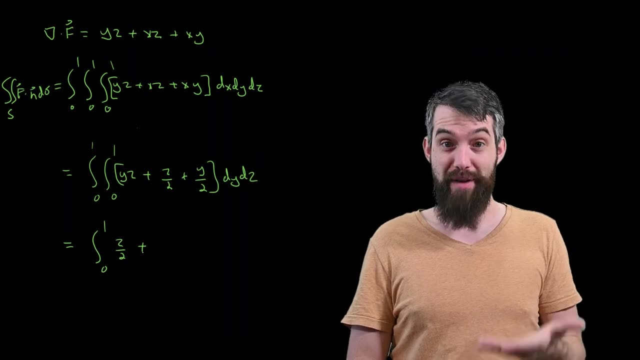 y squared over 2 times z. Plug in 0 and 1 into that and I'm going to get z divided by 2.. Then a z divided by 2 integrates to z divided by 2 times y. Plug in the 0 and 1, I just get z divided. 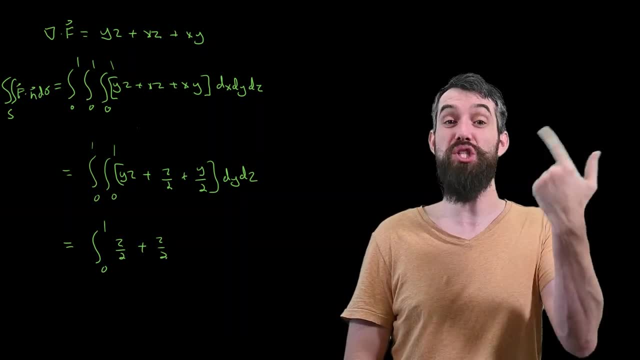 by 2.. And then the final term is y over 2 integrates to y squared over 4.. Plug in the 0 and the 1, and I'm going to get a 1 quarter, And then all of this is integrated with respect to z and. 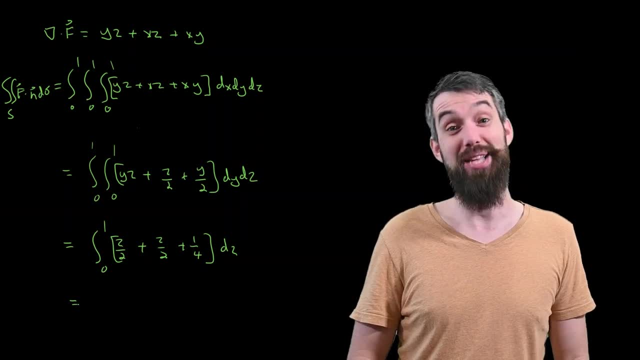 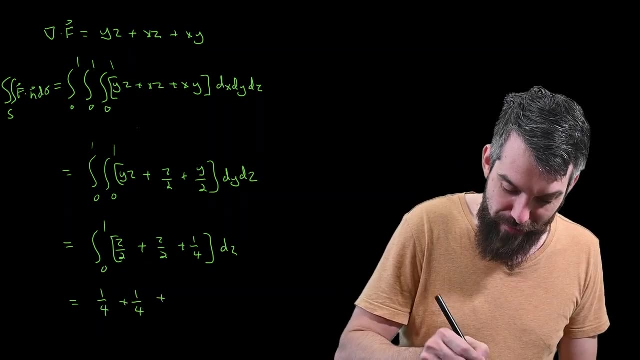 we're going to get our final answer very shortly here. So z over 2 goes to z squared over 4, so that's going to give me a value of a quarter. when I plug in the limits, Same thing, I have another quarter And a final quarter, and my final answer here is 3 quarters. So in this example, the 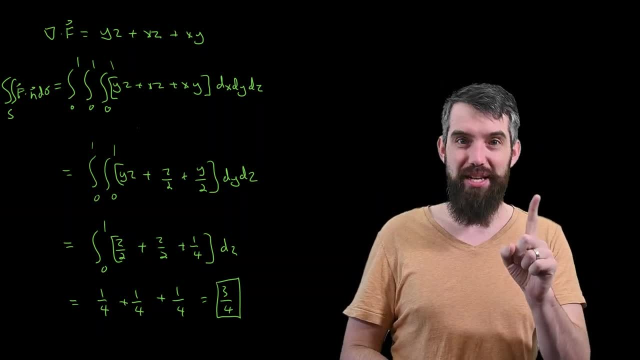 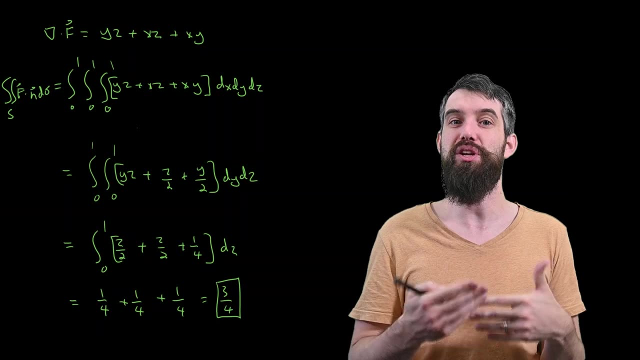 divergence theorem worked really well because we got the z divided by 2, and then we got the 1 integral. when we applied the divergence theorem- and we're going to use a triple integral- And it was a triple integral that we could do- It was easy to find out the limits of integration. 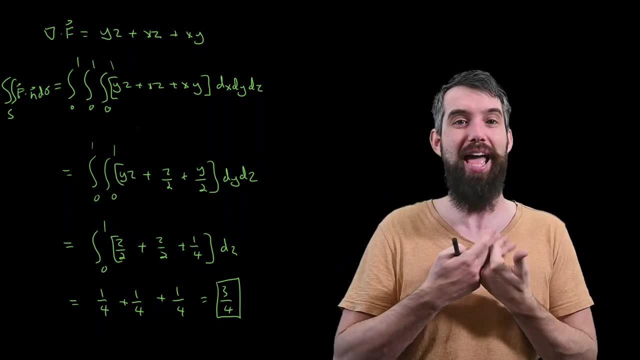 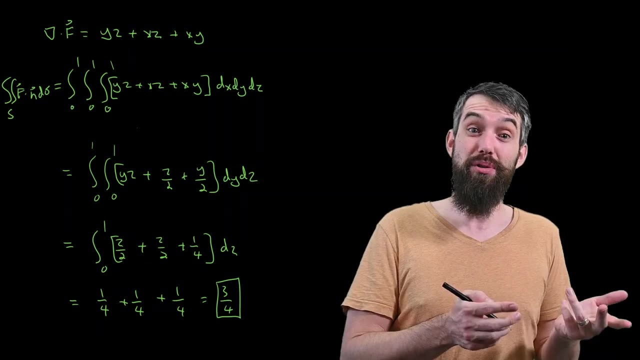 because it was just a unit cube that were all 0 up to 1. And so we could just execute that integration and we have finally found the outward flux across this blocks given by this particular field And, in general, whether you want to use the divergence theorem or just the standard old 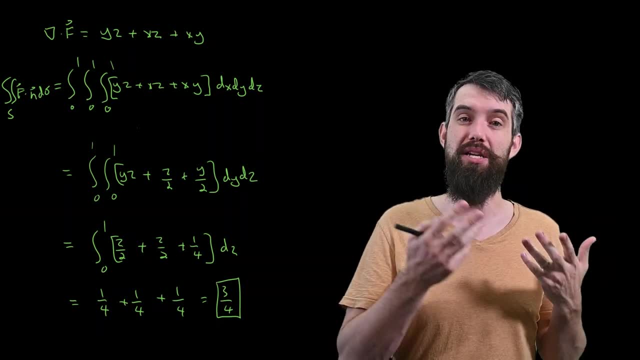 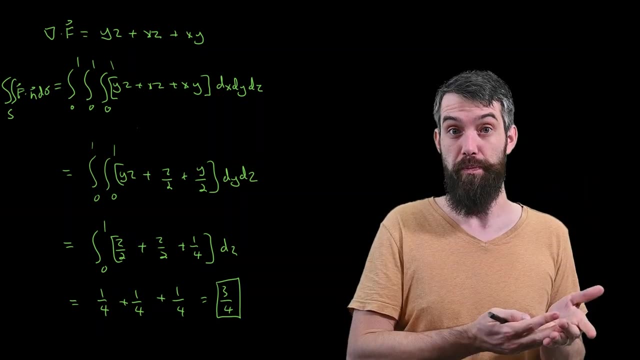 flux integrals that we've seen before just depends on the computational efficiency of the problem. If you can do the flux integrals without the divergence theorem, great. If it's easier to do with the divergence theorem, that's great too. All right, I hope you enjoyed this video. Please do give it a like for the YouTube algorithm, If you. 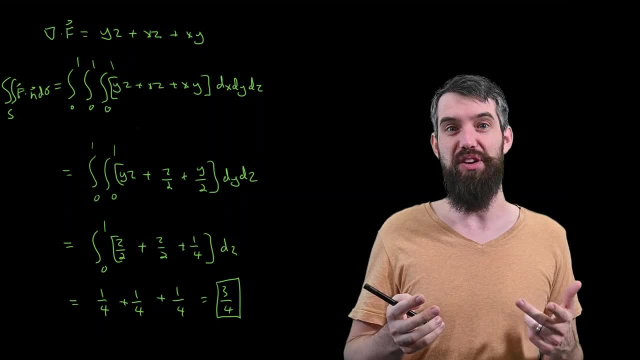 have any questions, leave them down in the comments below and we'll do some more math in the next video.